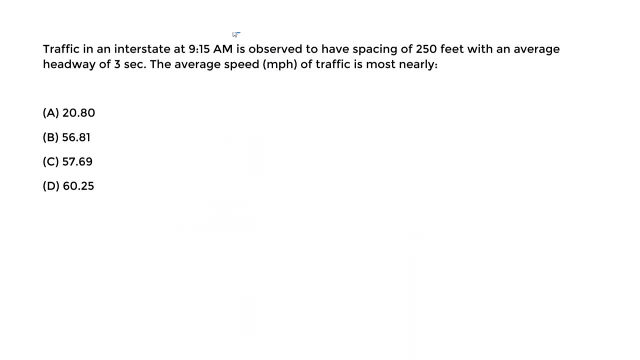 Okay, we have another example. Don't forget, pause the video. attempt this before you see me do the solution. So what we have here is a traffic flow or traffic stream parameter type question. So we're told here, traffic in an interstate at 9.15 am is observed to. 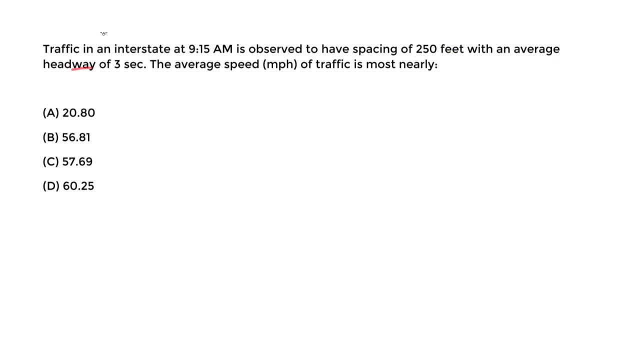 have spacing of 250 feet with an average head weight of 3 seconds. The average speed in miles per hour of traffic is most nearly what We want to find, the average speed. So let's state that as what we want to find Find. I'll call it AVG speed And let me give this: 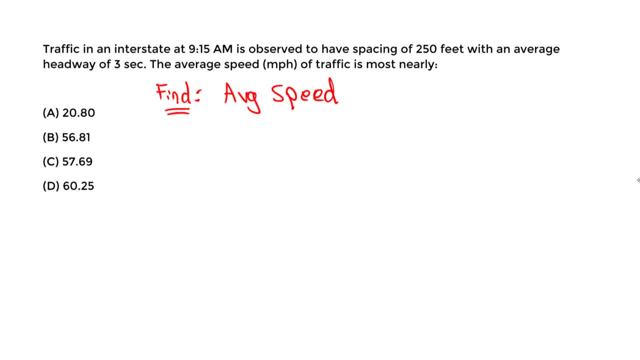 a variable and I'm going to stick with the FE handbook. right? We know some other books use very commonly. they use U for speed, So lowercase U for speed, but we're going to stick with the handbook and denote that by S. 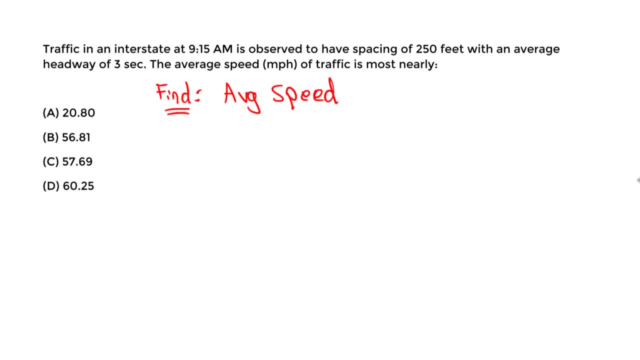 So let's use S and stick to the FE handbook, the NCS FE handbook. So we're going to find this S, the average S in this particular case. So we know we're given a few things here, So let's denote that. And we're given first thing: it's 9.15.. Okay, so that's irrelevant. 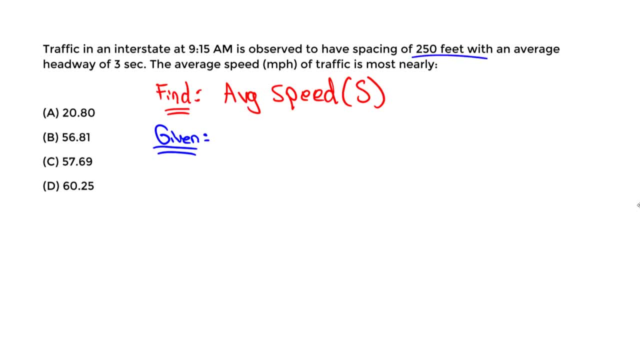 They just took that data at this time. So it's 250 feet of spacing. So spacing is a very, very important parameter when you're doing these things. So let's denote that by S traffic stream or flow analysis. These basic definitions are very important. So spacing: 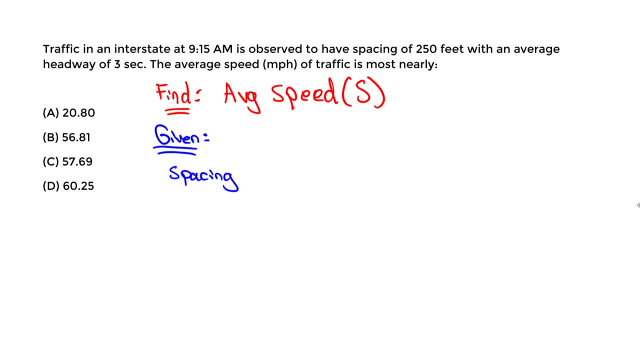 Spacing is going to be denoted by the lowercase S, So we'll give that lowercase s, as most books do, And we know that's 250 feet. 250 feet, Then the headway, the average headway. So this is the headway distance. Sorry, the headway time. Headway is not a distance, So 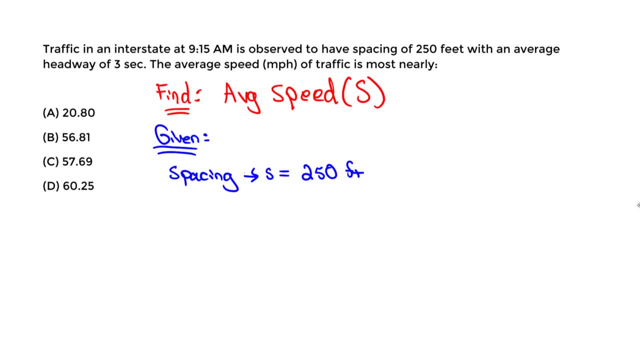 headway is going to be a time. spacing is related to headway, but we'll see that. we'll talk about that in the lesson notes. but just know, always stick with headway as a time. headway is always a time and in seconds, so seconds is the units we want as well. so the headway. let me write the. 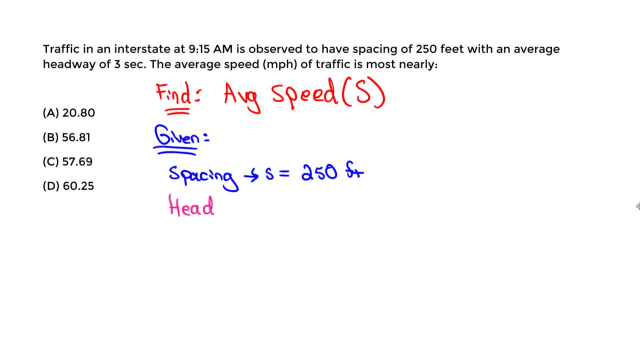 head way is going to be the lowercase h and this is the average headway. you can call it a h, sub average or we know we can do h bar. so you know, like when you put x bar, that's your like, mean or average, but that's the denotation is like that h bar is the average. so that is going to be. 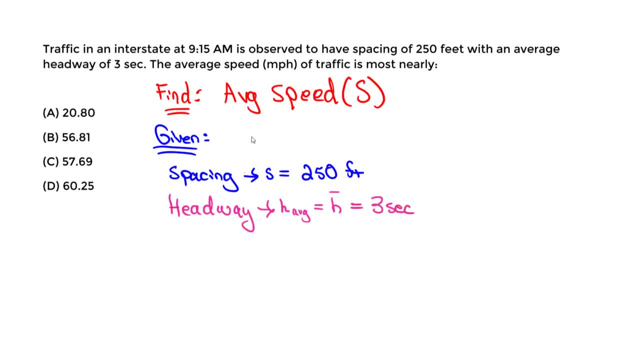 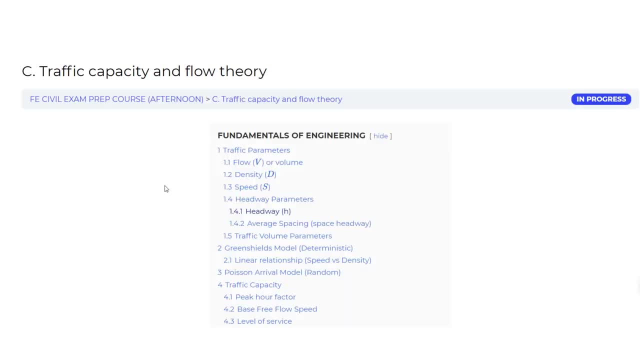 three seconds. so we have that and let's define these real quick. let's define these because we need to understand what these mean before we can solve this question. so if we look in the lesson notes, we know we have traffic parameters. so this is in traffic capacity and flow theory. so before we want to solve these, look at flow. 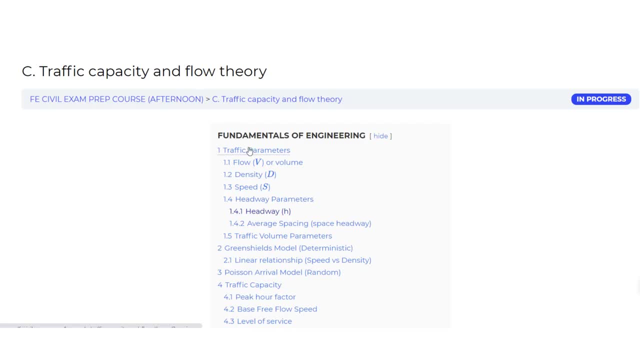 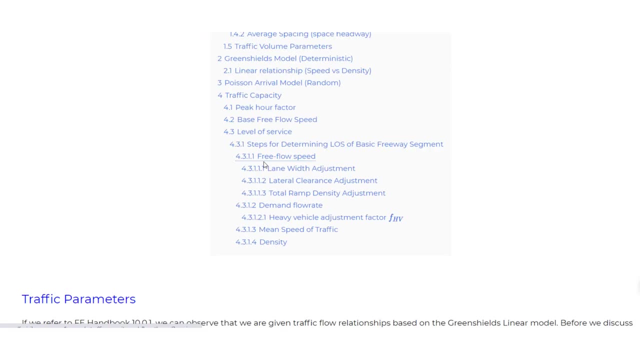 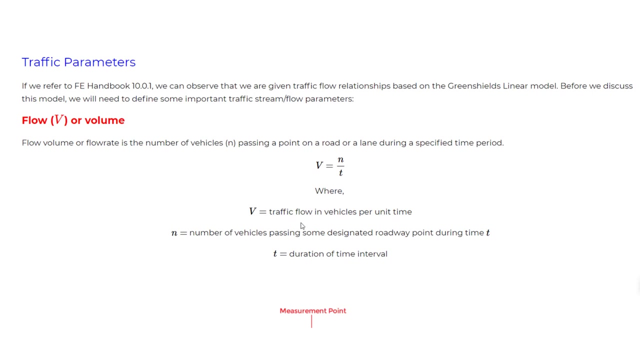 theories. we need to define these basic traffic parameters and understand what they mean. so traffic parameters we know in nodes. let me go above. we know like we define flow here. so flow, or the volume, is defined as n divided by t, and this is the number of vehicles passing a certain 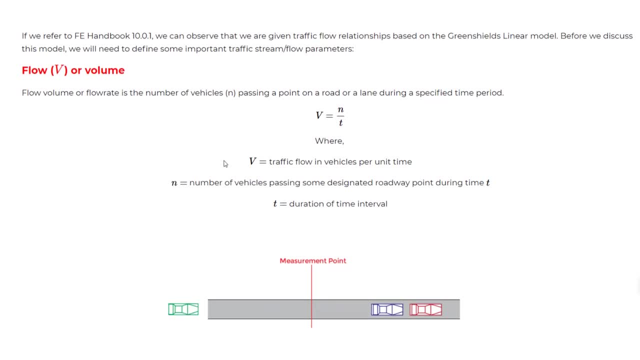 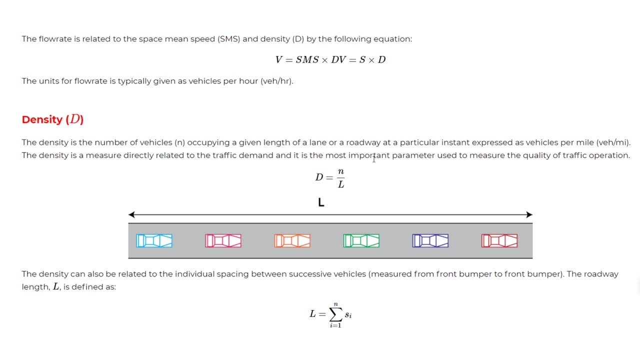 point per time. t is the duration of travel. so that's volume. then we define density is the number of vehicles passing a certain point per time. t is the duration of travel. is going to be the number of vehicles per length of roadway segment. we're analyzing. 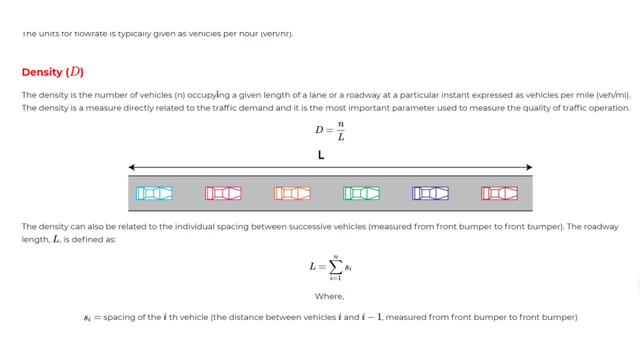 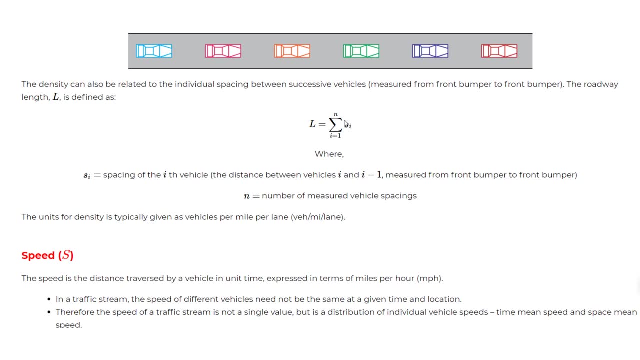 So that's going to be the density. So number of vehicles: n. n is the number of vehicles occupying the length. Then let's proceed. We know the length can also be denoted by this very important parameter called s. So s is going to be the individual spacing. 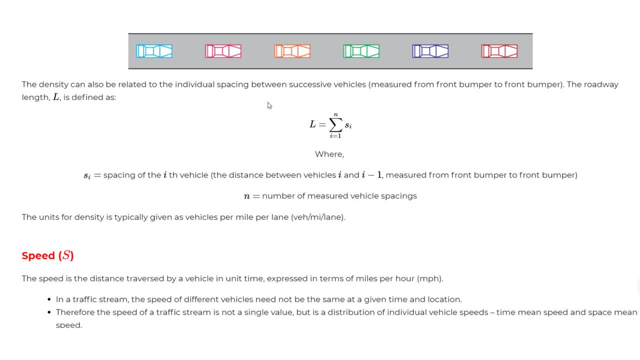 between successive vehicles, And that spacing actually can be related to the l value, the roadway length. So if we take the total spacing, successive spacing, which is like your average spacing, lowercase s, we can get the length of the roadway. So that makes sense. 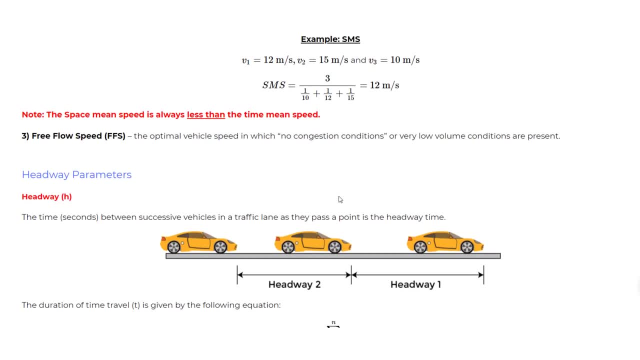 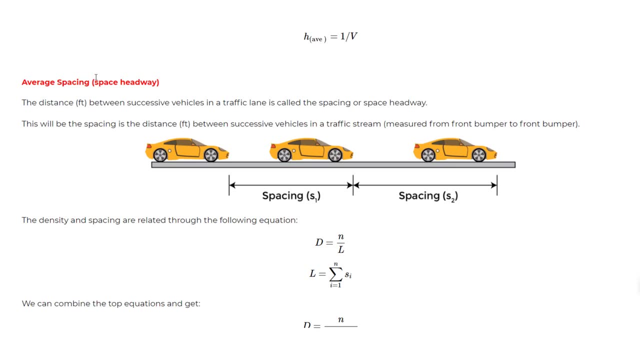 And that spacing. let me just jump into that, just to define that down here. The spacing is actually this average spacing. Some books use space headway but just know that spacing will have units of feet. It's not headway, Spacing is not headway. 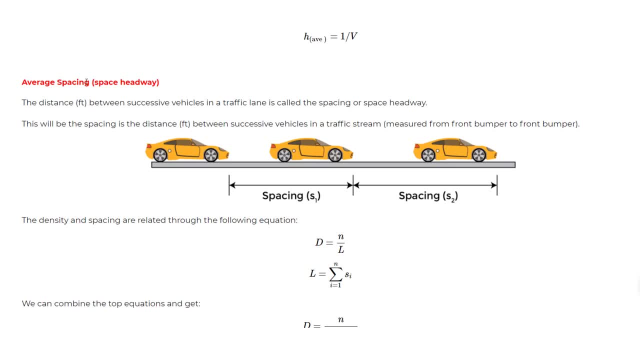 Headway has units of seconds, Spacing has units of feet And the spacing is like denoted here in the figure I provided for us, And it's from bumper to bumper. So this is the front bumper to the front bumper of this car. 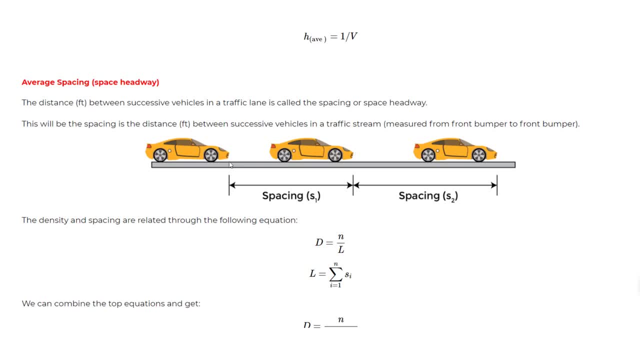 So the spacing s1,, for example, is from the front to the front of this. So that's what we mean by spacing And if you think about it logically, if you take the total summation of spacing, you take spacing 1. 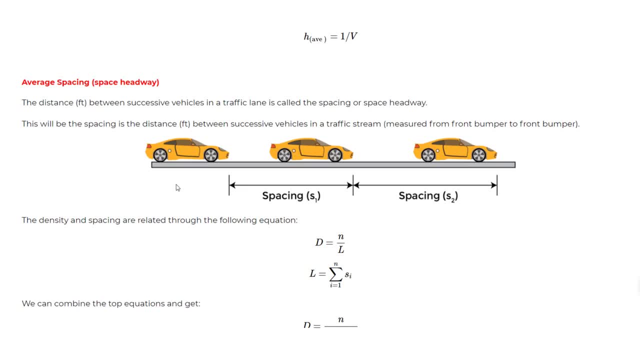 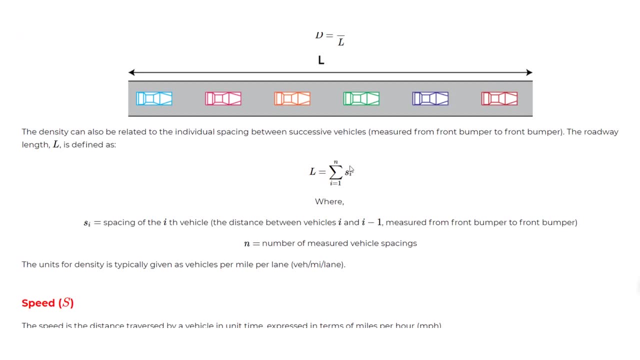 plus spacing 2, and you can arrive at your total length of the roadway, And this is where that comes from. This l, the total length of the roadway, is the summation of the spacing. This is a summation symbol saying start from vehicle 1. 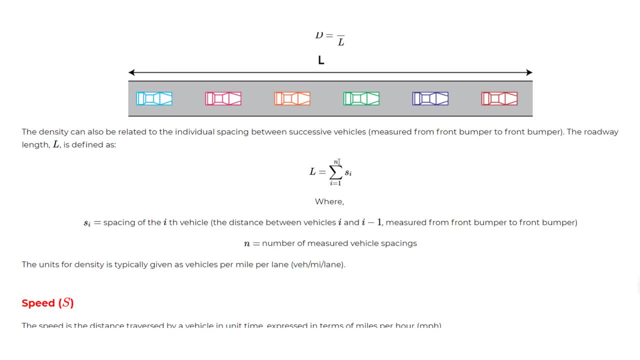 and go to n, how many vehicles you have, maybe five vehicles, So you'll have how many spacings. in that case, If you have five vehicles, you would have four spacings. You would have four spacings And then you just take it. 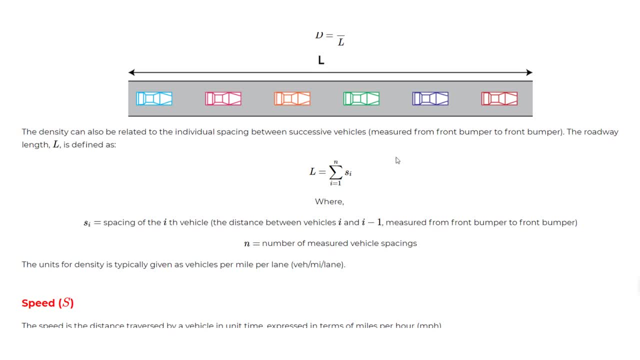 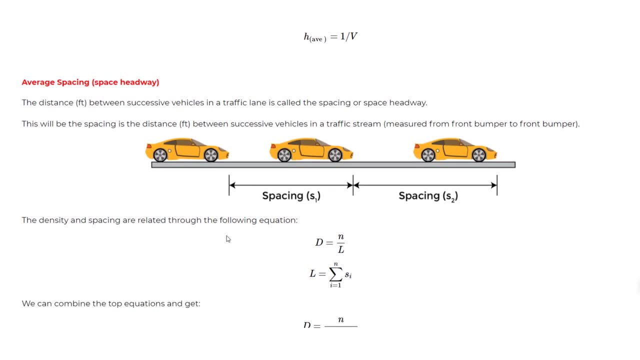 And then you just take the summation: So that's what this means, That's what that means. So then that's basically defining spaces. So we took care of that. We defined spacing. That's your average spacing, That's what they mean there. 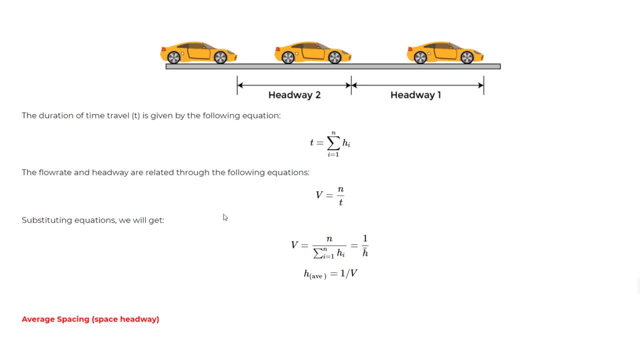 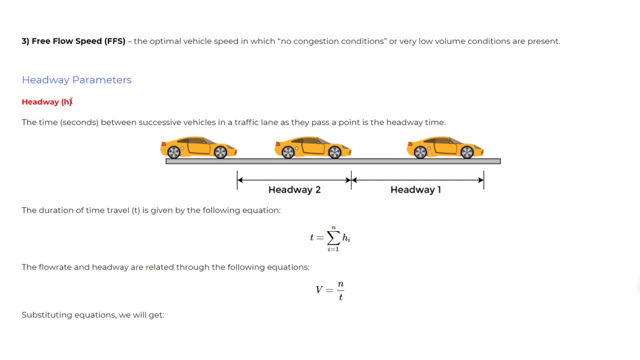 That's your average spacing, And then the other one is going to be what The headway? The headway is going to be lowercase h And again, headway is always units of time, So it's the time between successive vehicles. 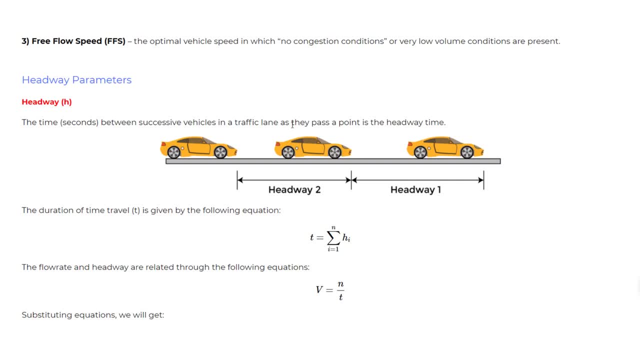 The vehicles in the traffic lane as they pass. a point is the headway time. So let's say we measure the point here, This car passes, Then this car would pass that point at a certain time right after that. But if you just use the figure here, 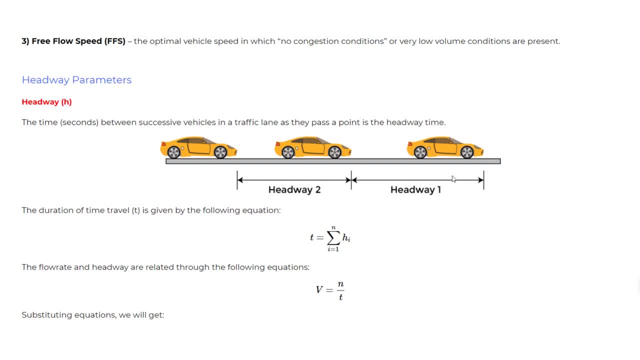 we know the headway between this and that is going to be that, Actually that distance the car needs to travel And we measure the time Right. We measure the time It needs to travel And that's going to be to travel this distance here. 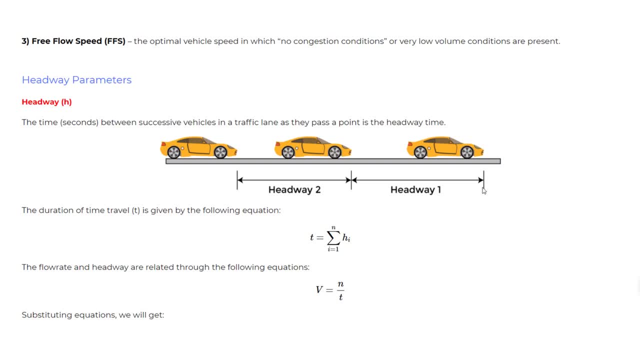 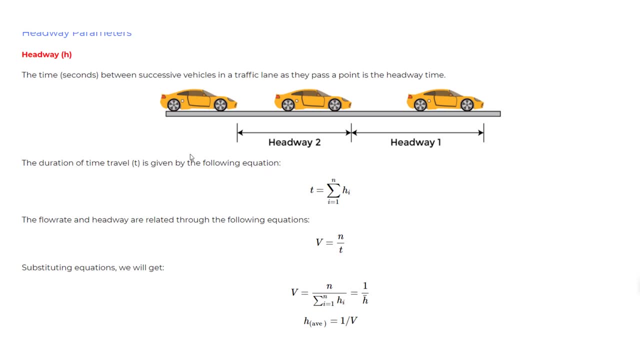 that dimension And that's going to be your headway. Headway is units of time in seconds, So we know that duration of time travel t is actually like your summation of the total headway time you have. This is the duration of time travel for a segment we analyze. 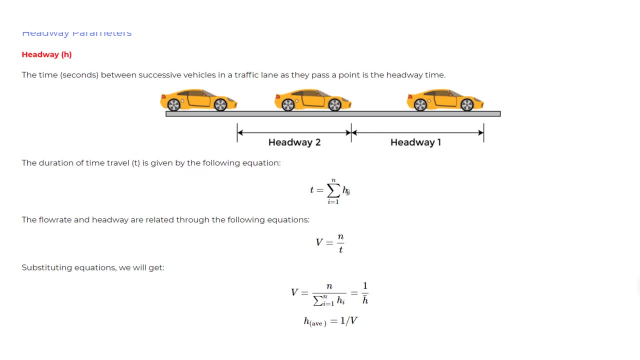 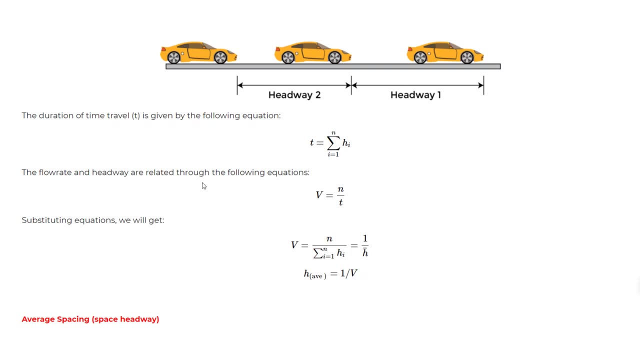 So we just sum, take the sum of the total headways. Again, lowercase h is the headway. That's the total duration of time travel for that segment we're analyzing. Then we know we can relate the flow rate to the headway. 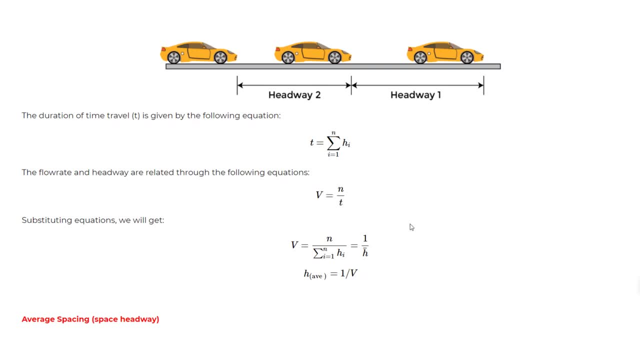 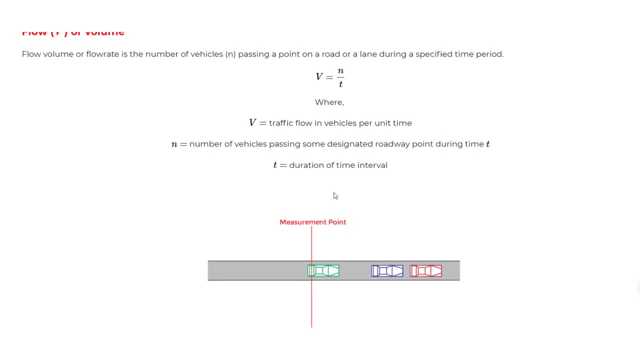 All we do is we know the flow rate. meaning is this: The flow rate v, not velocity. flow rate is v in the FE handbook is n over t, And that's at the very beginning right. v is n over t. 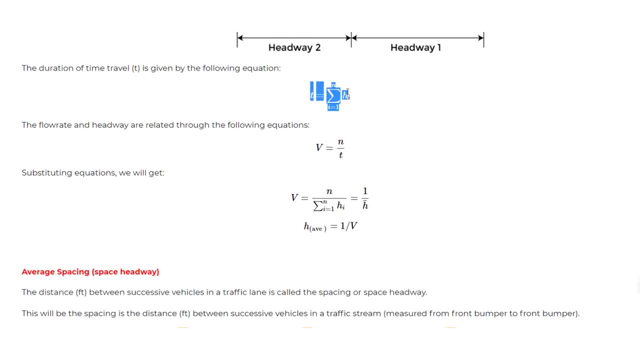 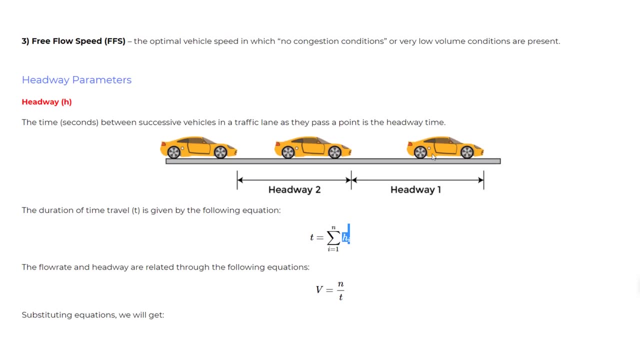 And that's going to be the flow rate. Then what we can do is take this t for the time duration, the total time duration of travel, which is, I'm going to say, t, Which is the summation of all the headways. 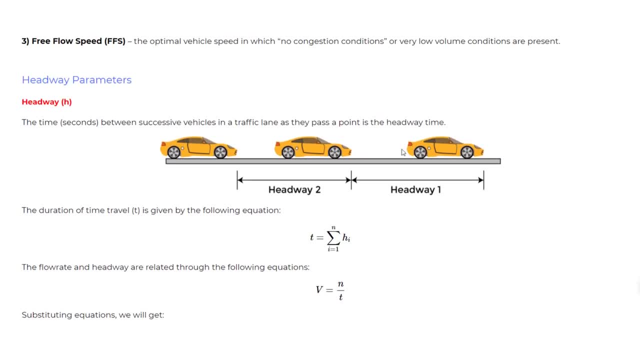 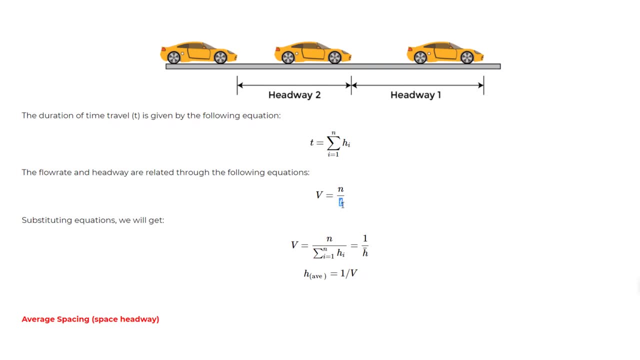 Let's say how many cars you have, You would do the total summation of the headway and that's your duration of time. So what we can do is take this t put it down here, and then we get this. Then we can arrive at this fundamental definition. 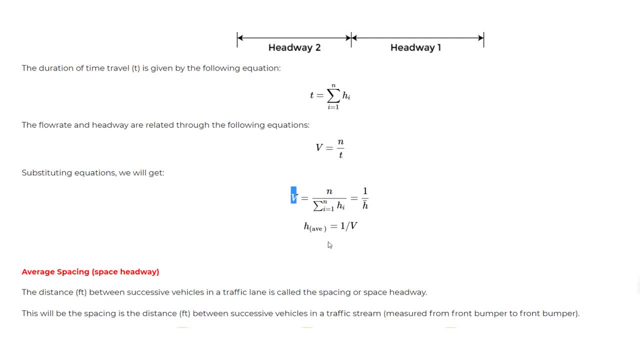 The flow rate is 1 over the headway, your average headway. So that's a very important definition that we can arrive at, which is actually not in the handbook, But I would honestly just memorize it and play around with it. 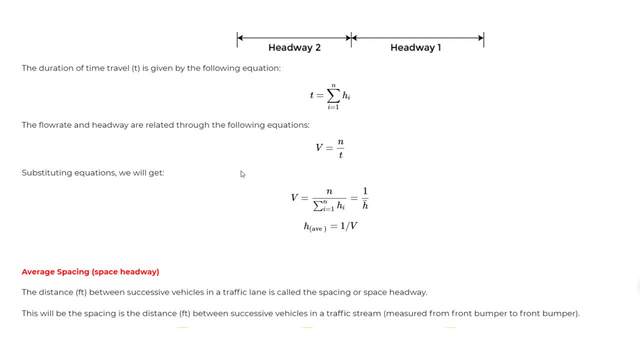 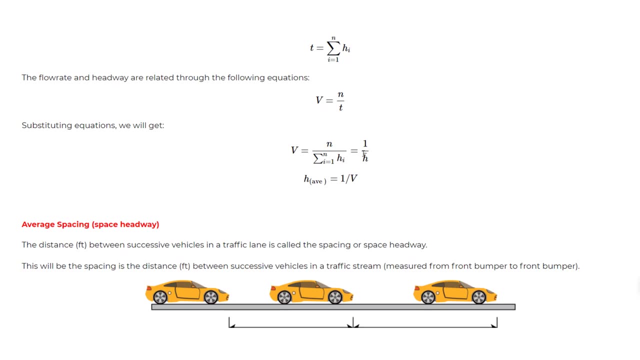 But on the FE, I believe they'll ask a simple question. Maybe they'll test your concept of headway, of spacing and so on. So we'll do examples just to get some practice in. Therefore, we can reorder this and solve. 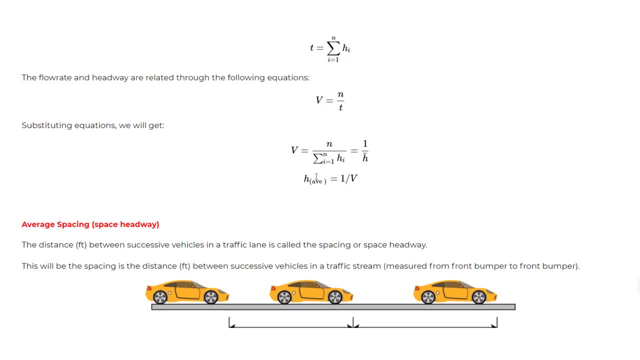 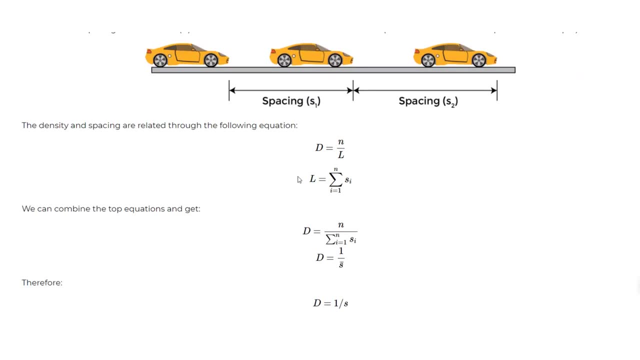 for the average headway, which is h bar average headway. This we get 1 over the flow rate. So that's also a very important definition. But I highly recommend you read over this and try to understand what each traffic stream parameter means. 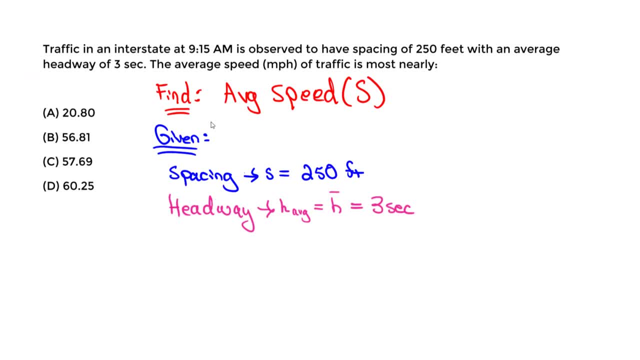 So that took some time, but we needed to know all of that in order to solve this question. So now we want to find the average speed. right, We want to find the average speed. So for the solution, let's dive into that solution now. 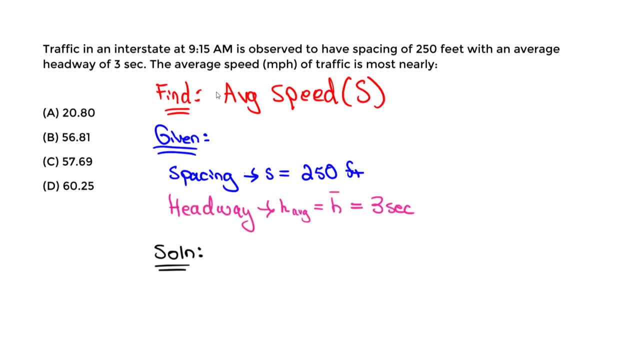 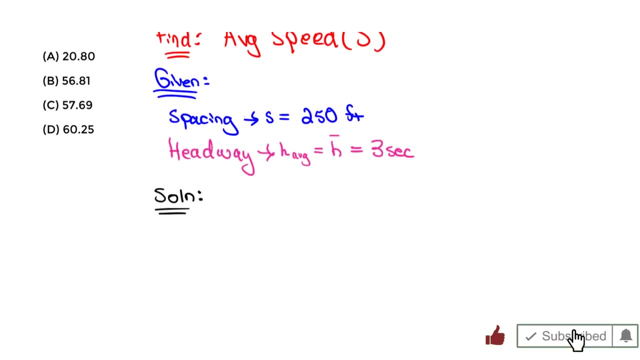 We know that the speed is something we can arrive at by actually using a fundamental definition. that's provided, I believe, in the FE handbook as well, And that's going to be the density. So what they wrote in the handbook on page 304,. 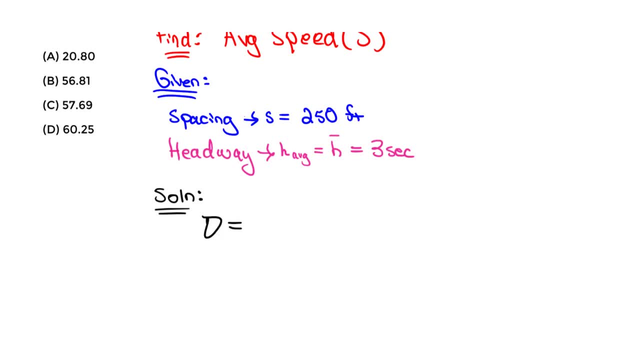 so pause the video, go to that page. the density is going to be your v over s, So that's in the handbook. They wrote italics v sub p. But just note that's the demand flow rate. But this is always true. 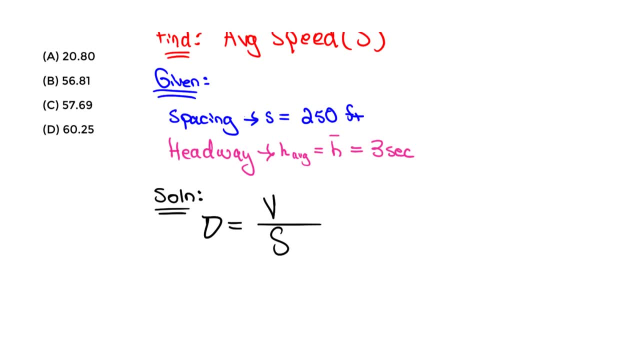 The density is the flow rate divided by your speed, And this speed is going to be the space mean speed, Space Mean speed, which is defined in the lesson notes. But anyway, we want to find that speed. This is how we're going to find and solve for that speed. 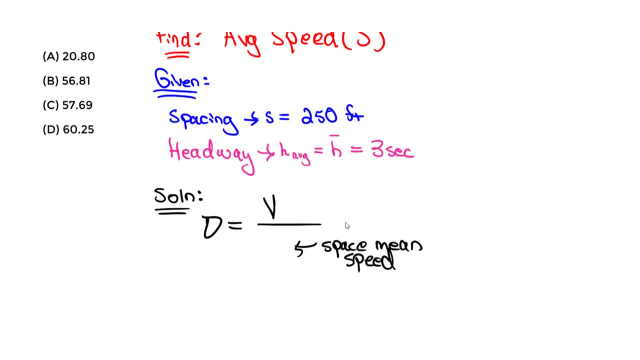 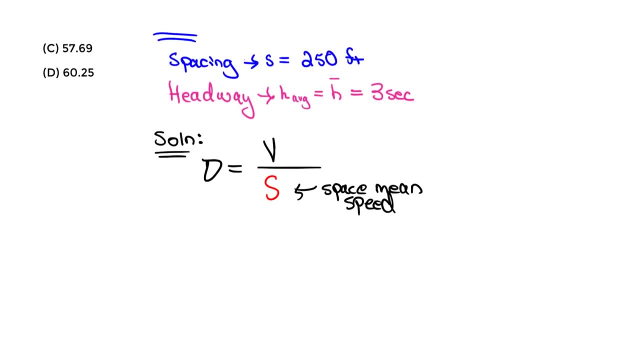 And let me give that red, Let me denote that by a red symbol for speed. We want to find that speed And that's the end goal: to find the speed. So this is the fundamental equation we're going to use, which is also provided in the lesson. 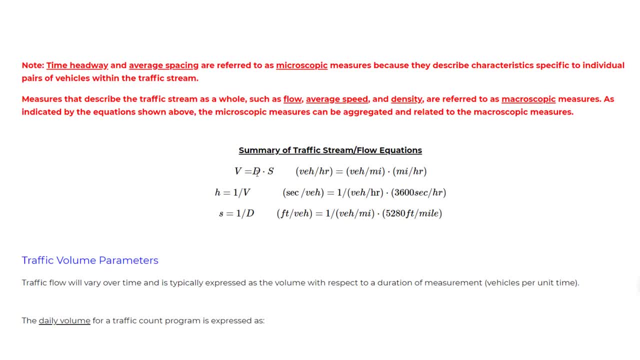 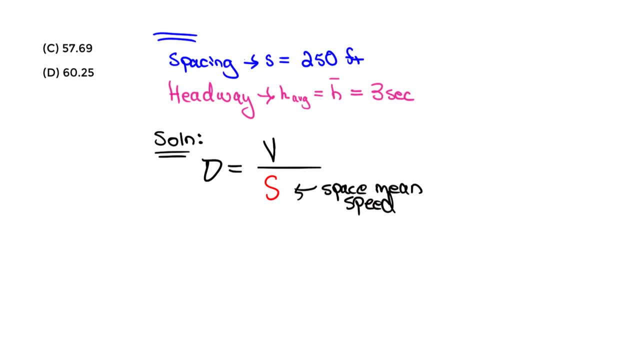 notes And we know it's basically this. We just rearrange that and solve for s right. That's all we're doing here. So that's going to be that equation. So then we're going to be like, OK, we're solving for speed. 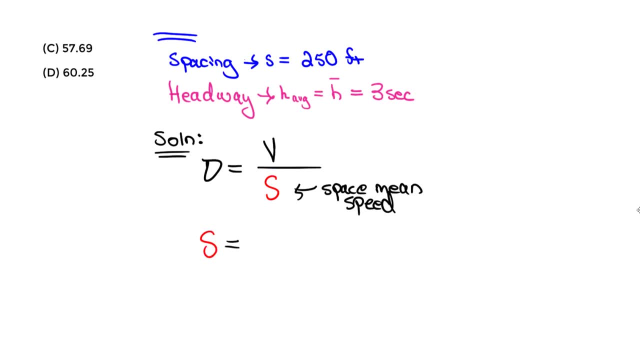 Let's rewrite this. Speed equals to what we take the v, which is the flow rate, divided by d, which is the density. So now, what we will do next is find the flow rate, find the density, Find the flow rate, find the density. 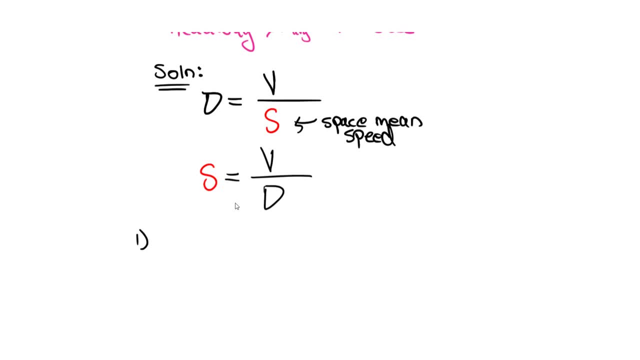 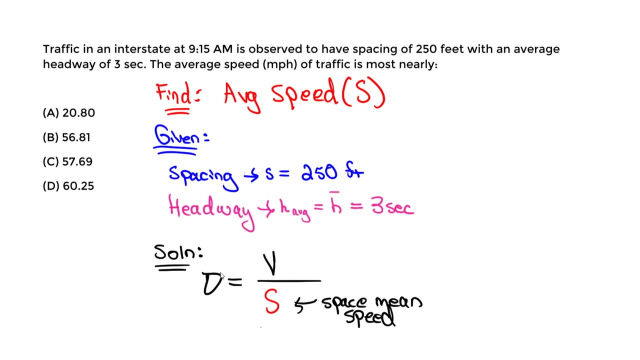 So we can calculate the density. Let's call this first step. We're going to say: calculate density by doing what? How can we find that density? We can find that density by using what we have here right, Based on these spacing and headway. 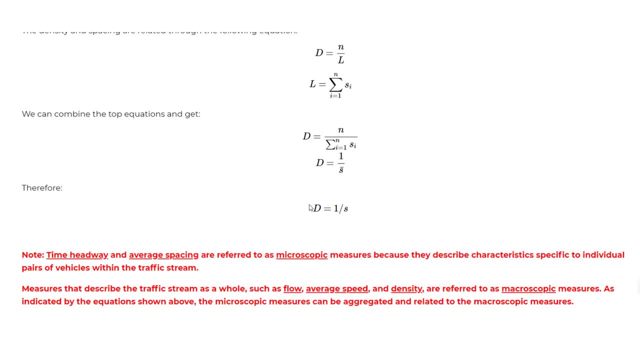 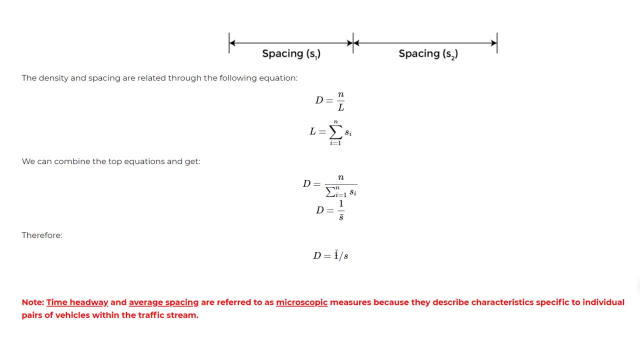 we can actually arrive at a density, Because we know the density is what. The density is always 1 over s. Density is always 1 over s. This is something you can memorize, especially for the fe right. You can. 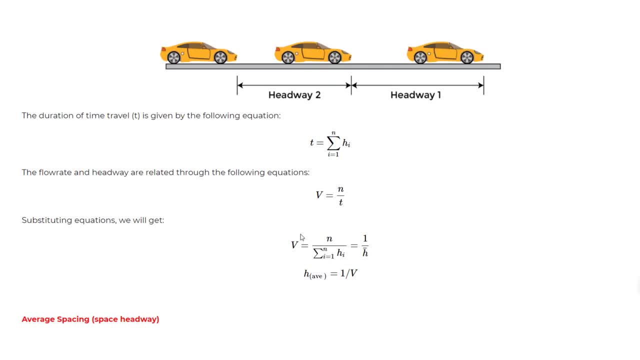 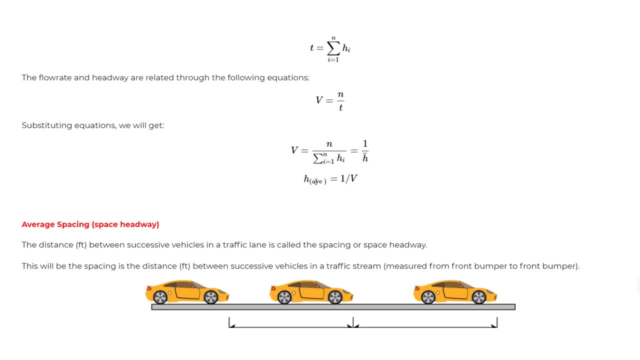 It's just 1 over s, always for the density, The flow rate. we know the headway is 1 over v. Be careful with that right. The h is 1 over v but density is 1 over s. 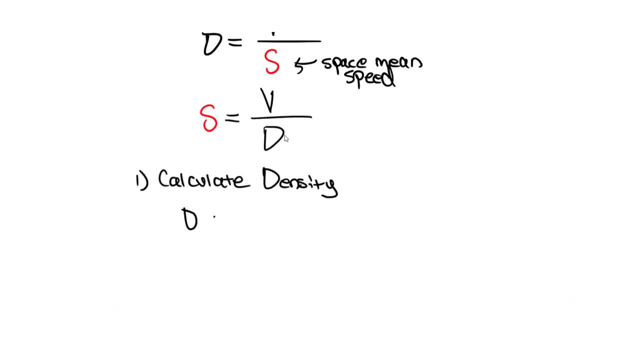 So let's write that Density equals 1 over s, where s is your average spacing. So this equals to 1 over Your s value here. That's given is 250 feet, 250 feet, But we know we want density in units always. 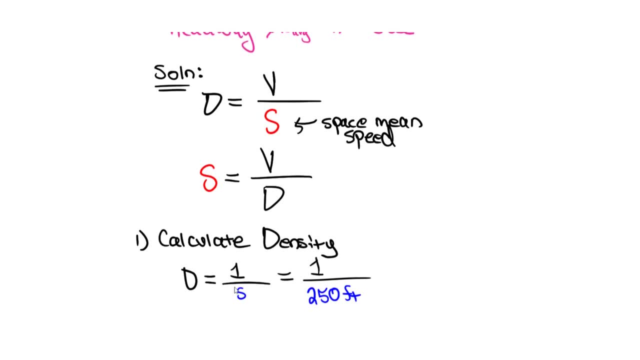 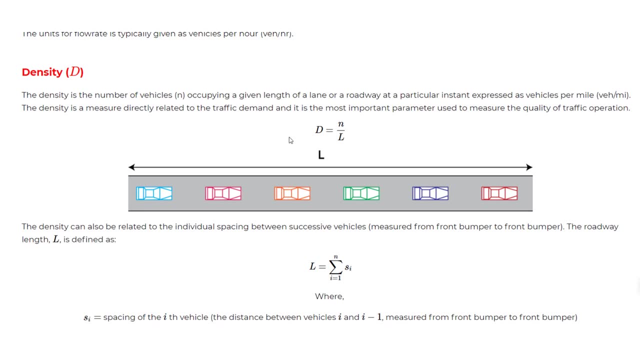 The conventional way to do this. when we're looking at US units, which is what's expected on the fe units of what? What's the units of density, We go above. Density is defined in units of vehicle per mile per lane. 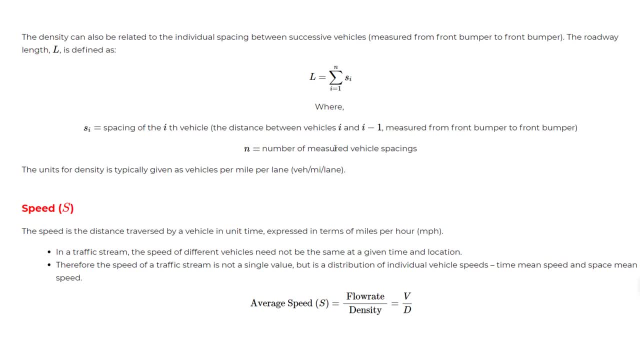 Typically like vehicle per mile and usually we're only looking at one lane right Or one roadway segment, So it's vehicle per mile per lane. Vehicle per mile: always Vehicle per mile per lane And typically the data is per lane. 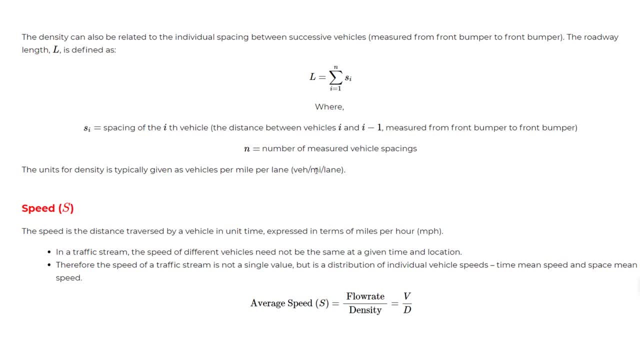 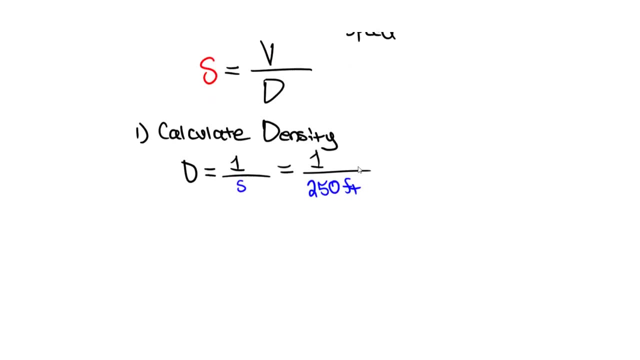 So that you can just eliminate. But vehicle per mile, it's always the vehicles on top per mile right. Vehicles per length, So that's going to be the units for density. So let's reduce this and take out that. feet right. 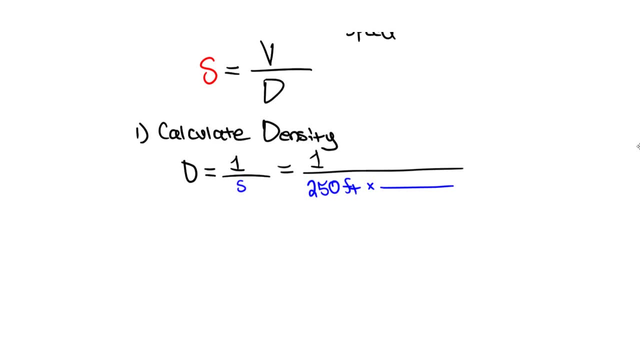 And convert it to miles. So we know that there's going to be how many feet in one mile. So this is going to be important. It's 528.8.. 5,280 feet in one mile And this is in the tables at the beginning of the FE handbook. 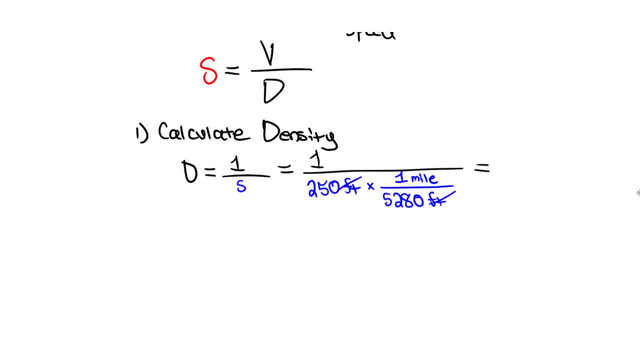 So these cancel. So now we can solve for the density. So, solving for that density, we get the times 1 over 5,280.. We should get about 21.12.. So that's the density. So that's going to be the units of vehicle per mile. 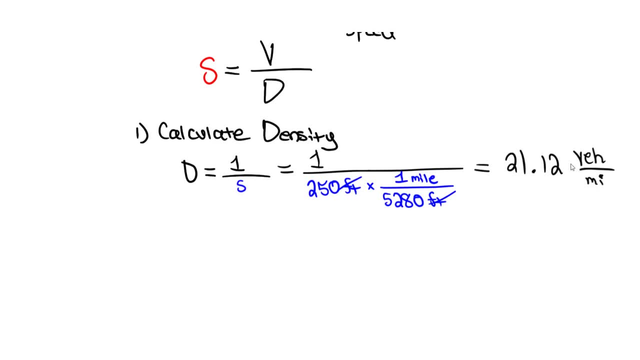 So we have that Now. we can now proceed to finding the flow. So we can next find the flow, Let's say calculate flow rate. And for the flow rate, we know that definition is what. The definition that we will use is the one with respect. 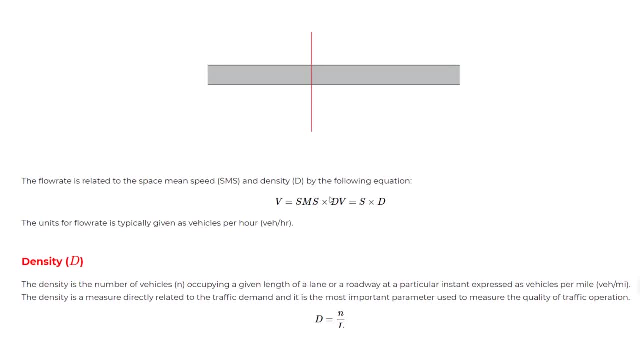 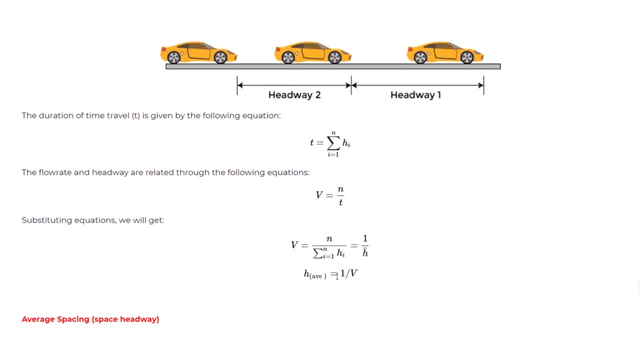 to the headway right, Because we know the headway and that's actually given. So if we go we know the headway. down here under headway parameters The headway is always 1 over v right, 1 over the flow rate or the volume. 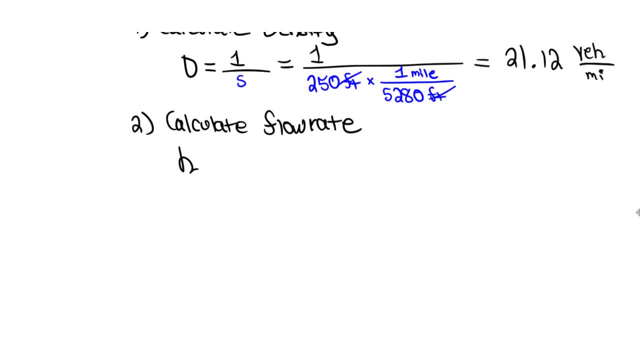 So we know the traffic volume. So the headway. what color did I use above for the headway? This right, I'll call it h bar. h bar equals 1 over the traffic volume. So we can solve for v: v equals what? 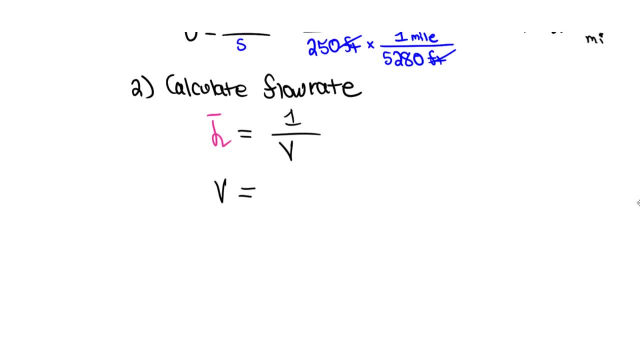 1 over the headway. 1 over the headway. So then that equals to 1 over the headway. we said is how many seconds? It's 3 seconds, right, 3 seconds, And you have to be careful with this, the units here. 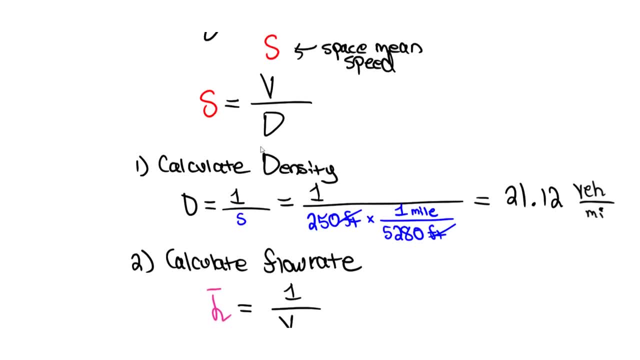 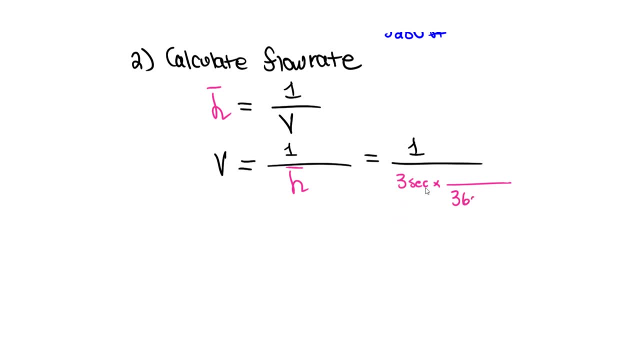 They'll trick you on the FE And we know we need units of what Hours, right Miles per hour. So let's take out the seconds And convert it to hours. We know there's 3,600 seconds in 1 hour. 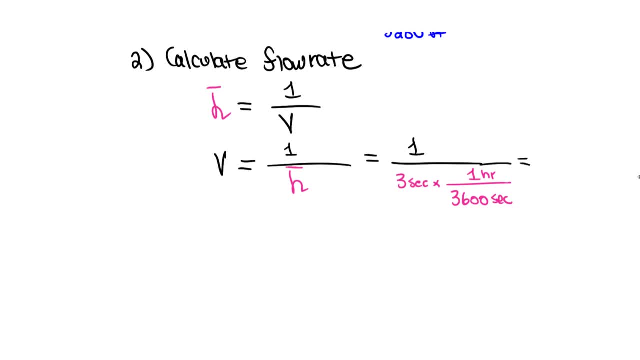 This is always true, right? You should try to memorize that That's an important one. So these cancel. You do 1 over 3 times 1 over 3,600.. And you get 1,200.. You get 1,200. 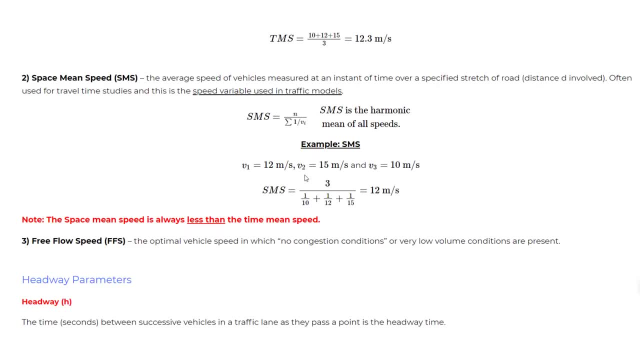 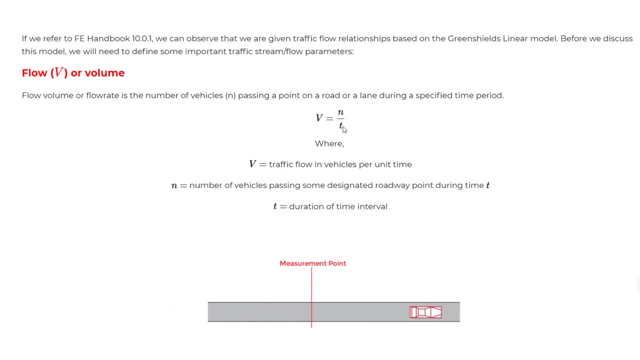 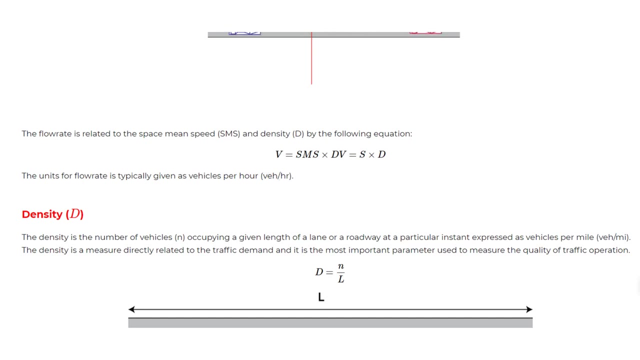 And the units for flow. the units for flow are what It's: the flow. So the very first units are going to be vehicles per time, Right, Vehicles per time. So the vehicles per time is going to be vehicles per hour And that's the typical units for when we're working with US. 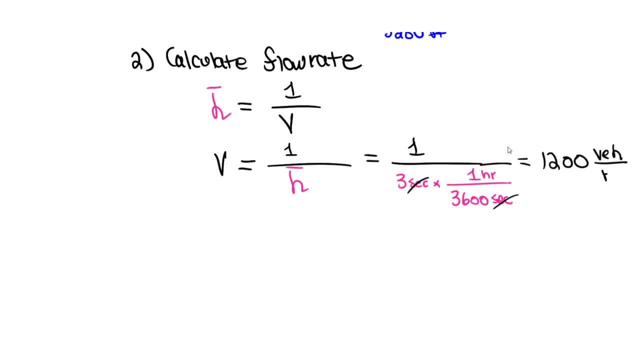 or English units. So vehicles per hour is always what we want. So now you have all of that. We just plug it back in here and solve for the speed. Speed equals to what We take the density. Sorry, we take the flow rate divided by the density. 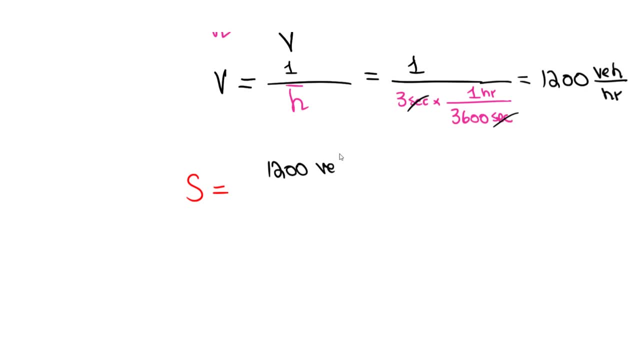 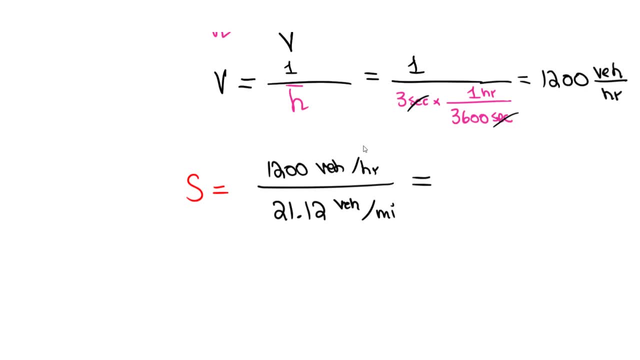 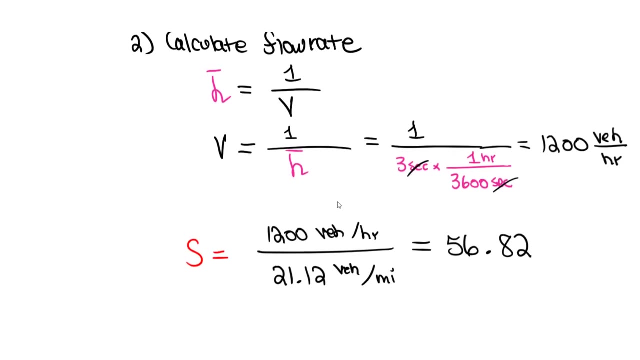 So you do 1,200 divided by 21.12.. You get about 56.82.. And we know the vehicles, So we have units of what for the speed? So it's going to be miles per hour, right, So we know the vehicles. cancel miles per hour.